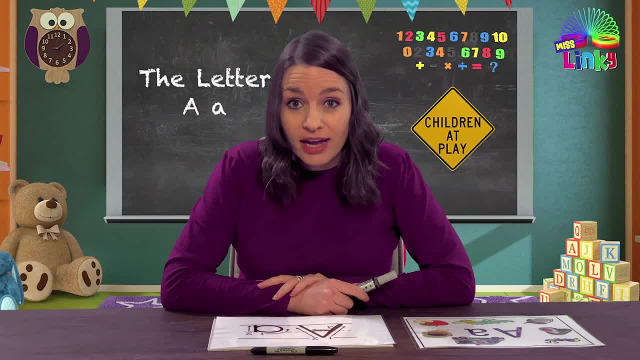 Now, here we are going to write the capital letter A. Let's try it one more time: Down, down and across, And there you have an uppercase letter A. Can you see that it looks a little bit like a triangle. You have to practice writing this until you get it right And remember the more you. 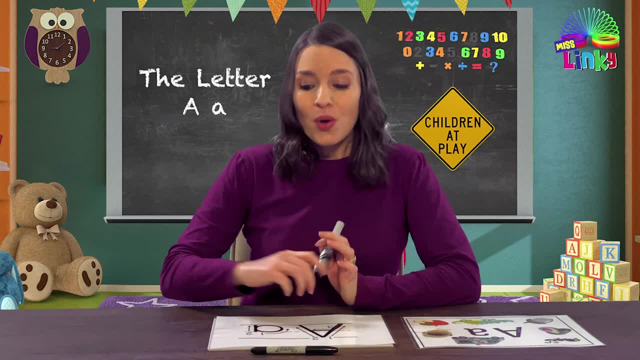 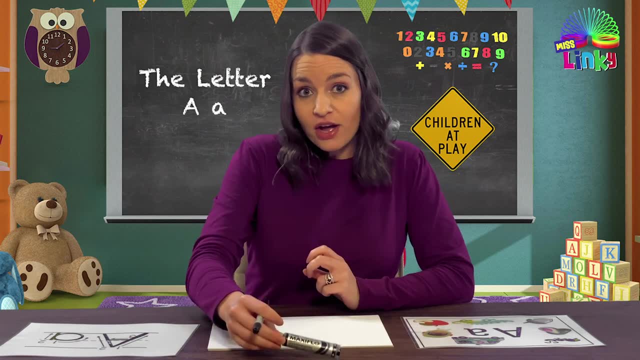 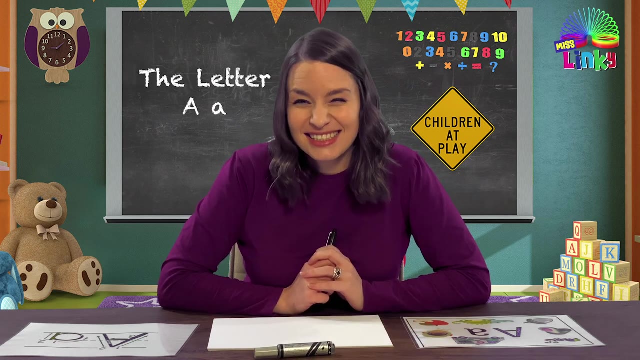 practice, the better you will get. Now we're going to play a game. For this game, I am going to draw a picture that starts with the letter A and you are going to guess what it is. Are you ready? Yes, Okay, let's go Now. watch carefully. 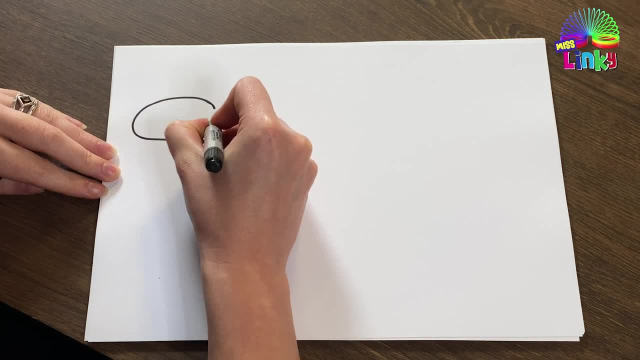 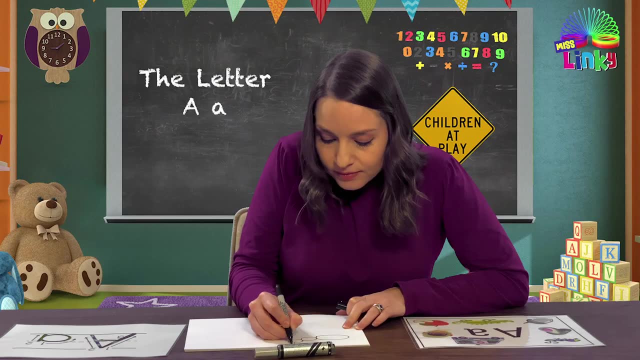 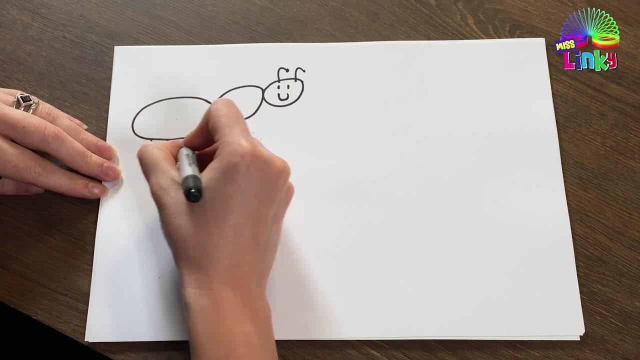 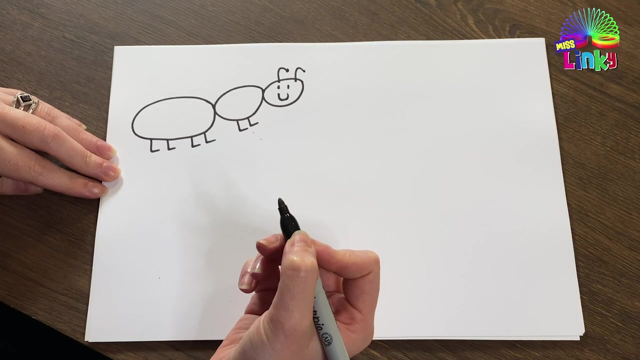 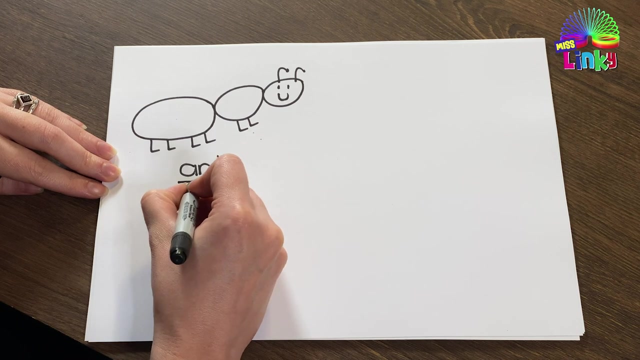 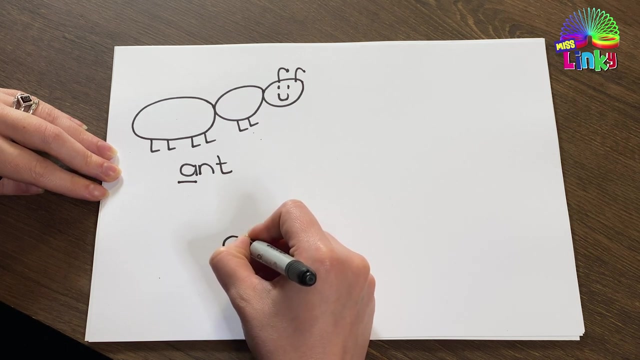 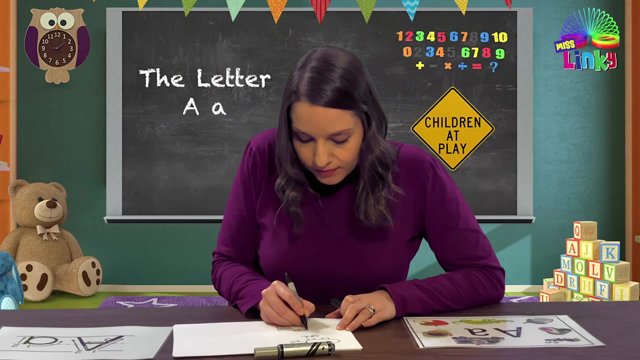 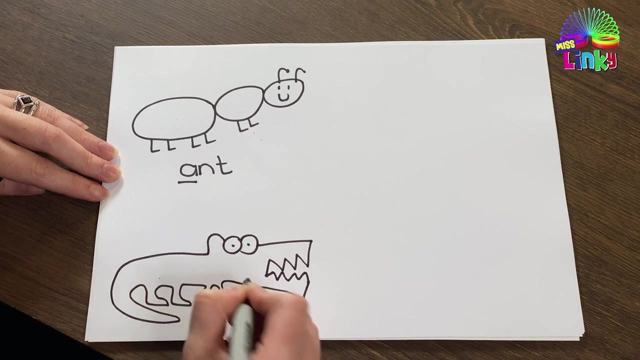 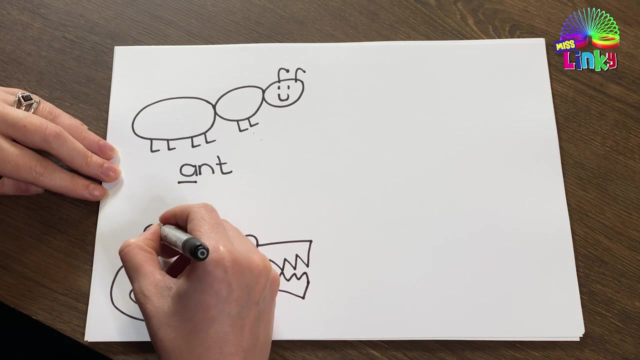 Do you know what that is? That's right, It's an ant Ant Ant stop. Do you know what that is? That's right, It's an ant Ant Ant stop. starts with the letter A. Let's do another one. Can you guess what that is? It's an alligator. 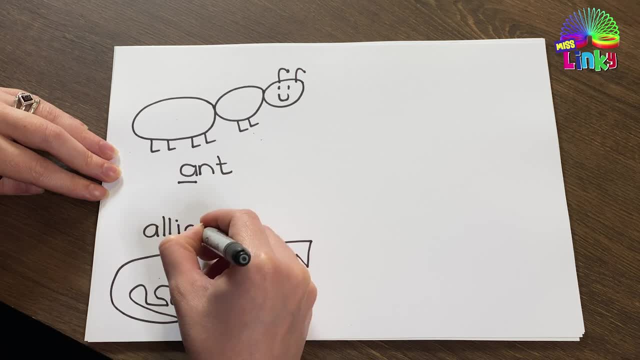 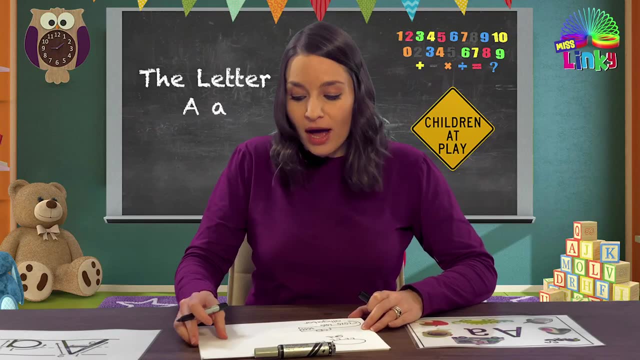 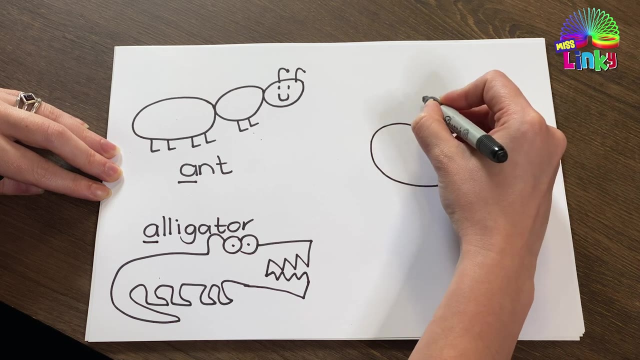 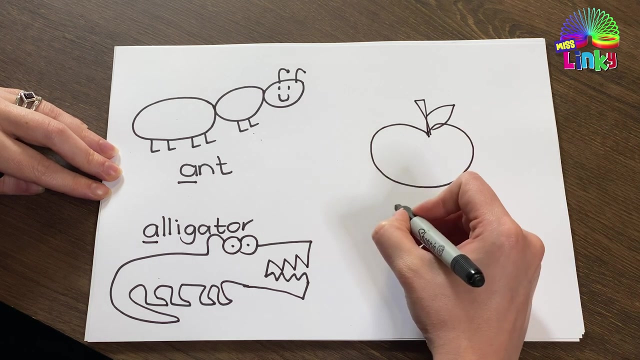 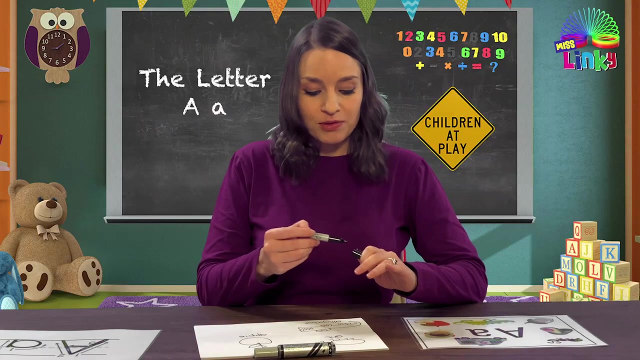 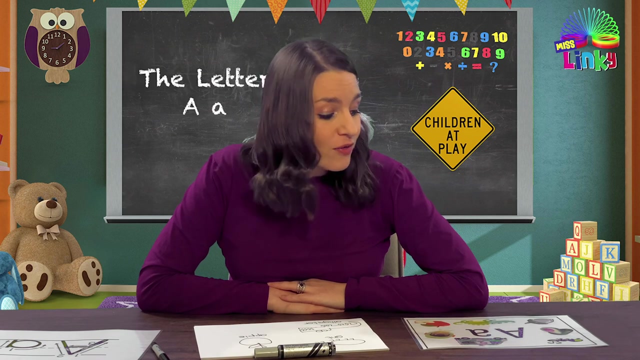 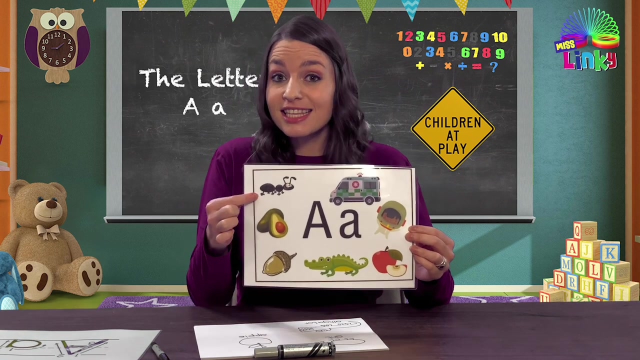 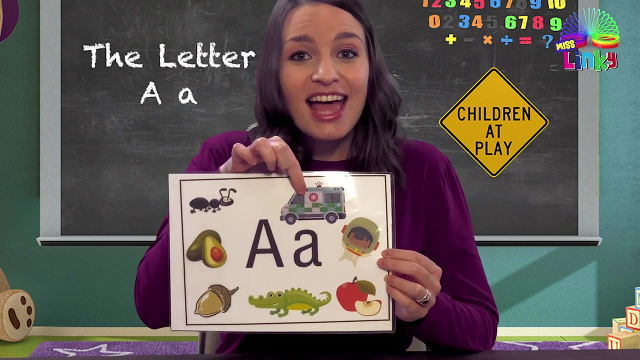 Alligator. Alligator starts with the letter A. Good job, And let's do one more. Do you know what that is? That's right, It's an apple. I love apples. How about you? Do you like apples? Good Apples are healthy. Now we are going to look at some pictures that start with the letter A, And I want to see if you can name the things in the pictures. All right, Here we go. So we already did this one. It's an ant. This is an ambulance- Very good.